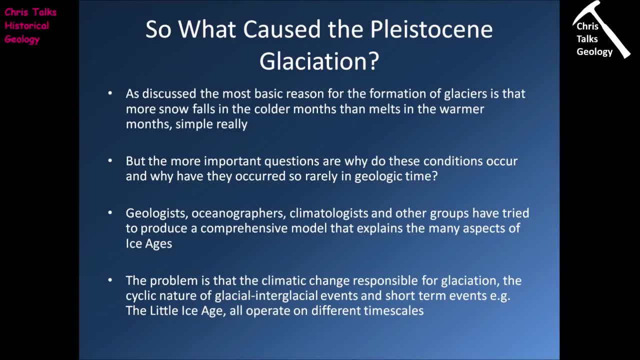 that's Greenland. Please make sure you write that down, put it somewhere safe, because you'll need it for the code word quiz. So now we need to think about what actually caused the Pleistocene glaciation. Now, as discussed, the most basic reason for the formation of glaciers is that you. 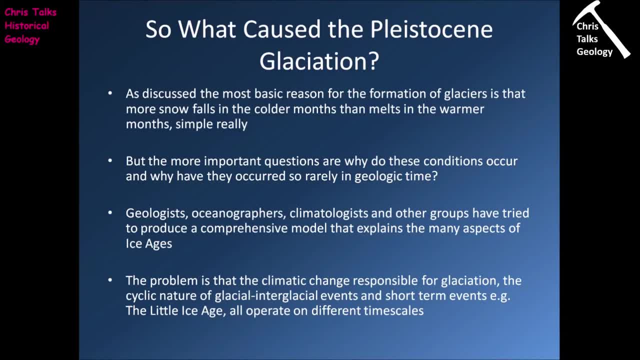 get more snowfalls in colder months than melts in the warmer months, so you have a net build-up of snow and ice. But the more important questions are: why do these conditions occur, and why have they actually occurred so rarely in geologic time? So when you think about it, we don't actually have 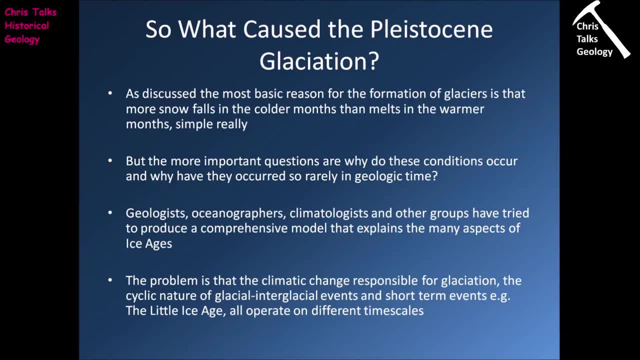 many examples of these large-scale glaciation. So we know we have large glaciations at the end of the Proterozoic. we know we also have large glaciations occurring during the Carboniferous and we know we have these large-scale glaciation occurring as part of the. 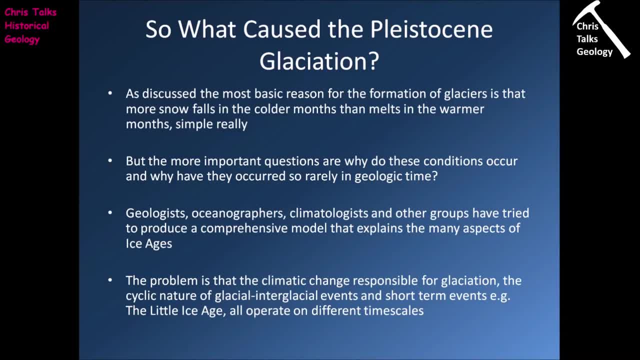 last ice age, But in between those events there are huge amounts of geologic time where we don't have these glacial events, and so this is showing us that the conditions that lead to the formation of large glaciers, large glacial events, are obviously relevant. 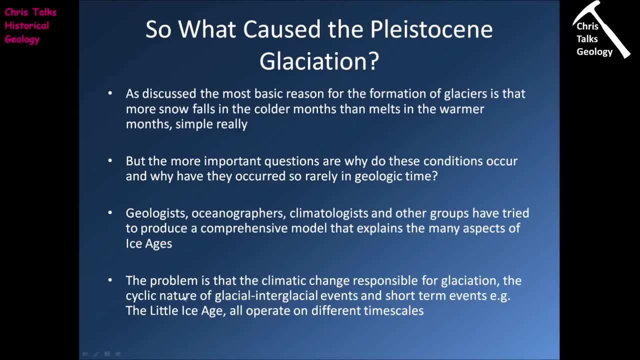 So the problem is is that the climatic change responsible for glaciation and the cyclical nature of glacial interglacial events and the additional complication of short-term events, all operate on different time scales, And so we have lots and lots of different processes occurring. they're all 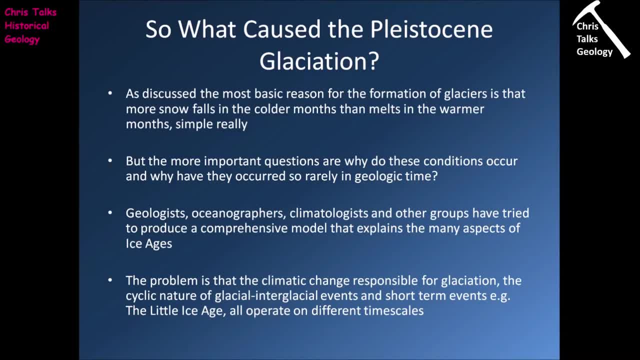 operating on different wavelengths, essentially, and so this means that the chances of you getting all these different factors to occur are relatively low, And so this makes it less likely you're going to get these glacial events. So the question then becomes is: well, what are the conditions we're looking for? 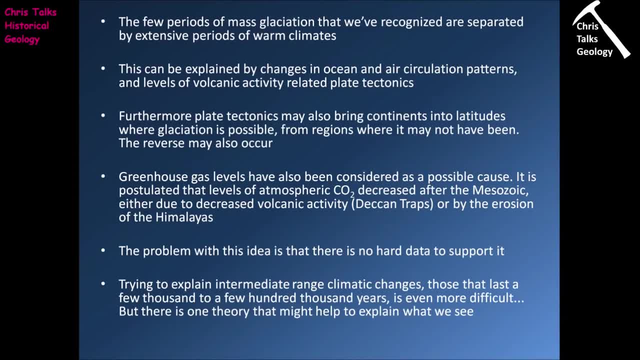 in order to encourage the formation of large amounts of glacial ice. Now, the few periods of mass glaciation that we've recognized are separated by extensive periods of warmer climates. Now this can be explained by changes in ocean and air circulation patterns and levels of volcanic activity. So that's obviously going to have a serious effect. 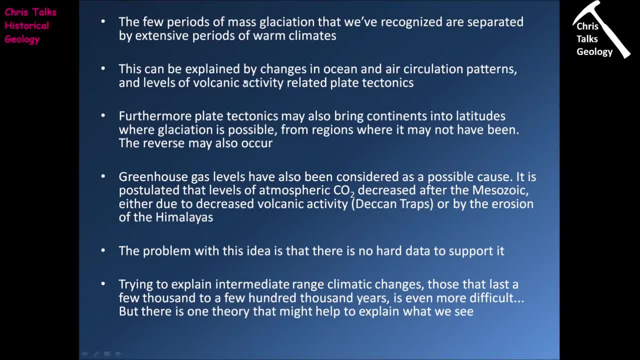 on greenhouse gases and thereby it's going to cause an increased or decreased greenhouse effect. Typically, when we have lots of volcanic activity, more carbon dioxide enters the atmosphere and the greenhouse effects become stronger, and this is obviously going to inhibit the formation of large amounts of glacial ice. Now, furthermore, we know that plate tectonics may also bring continents. 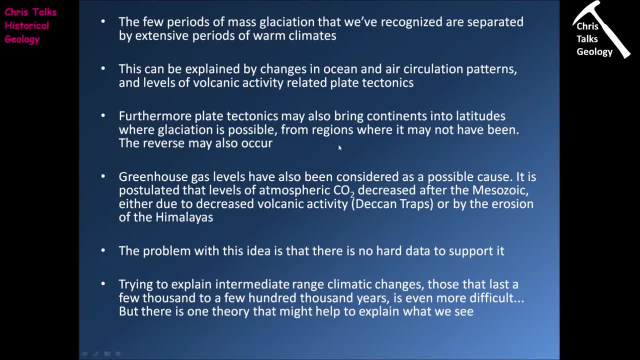 into latitudes where glacial events are less likely to occur, So this is obviously going to have a higher chance of forming large amounts of glacial ice. So if you go and distribute all of your continents along the equator well, that's obviously going to mean that the chances of you having an 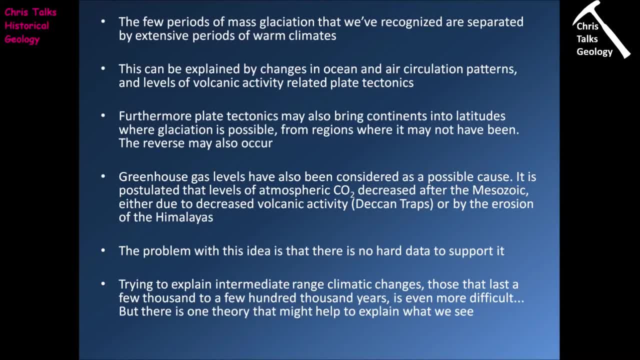 ice age are reduced because it's more difficult to form glacial ice in tropical regions. In contrast, if you were to push all the continents towards the poles, well, that would obviously displace warm sea water with cold water and that would reduce the chance of forming glacial ice. 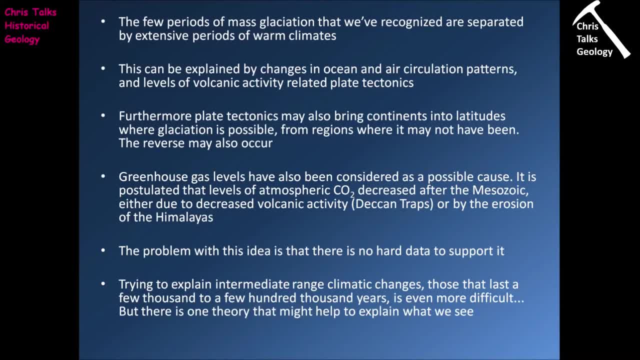 Water with cold continental crust, and so that would encourage the formation of ice sheets, both because the continental crust has moved into areas which are essentially because the continental crust will encourage the nucleation of ice, and it's been pushed into areas which are naturally more cold. And so, on the very first level, what we are looking for is a decreased 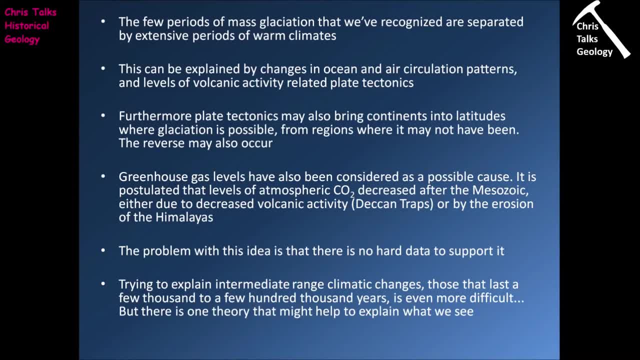 greenhouse effect, because that's going to help to drive down global temperatures, and we want crust to be located near or at the poles. So those are the first couple of conditions which we want Now. greenhouse gas levels are often considered to be a possible cause for glaciations. 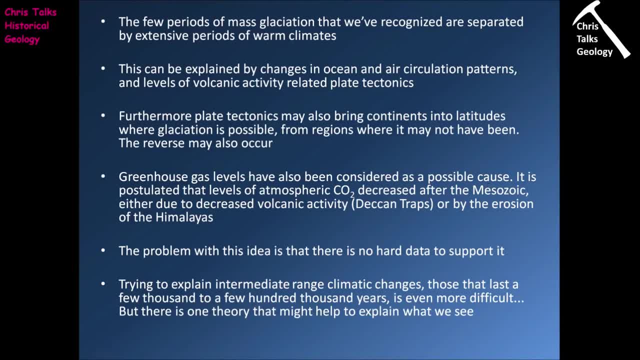 You know it makes a reasonable amount of sense. when greenhouse gas levels are low, the greenhouse effect is going to be weaker and the global climate will therefore be cooler. And you know, given the right conditions, this could lead to the onset of a glacial event. 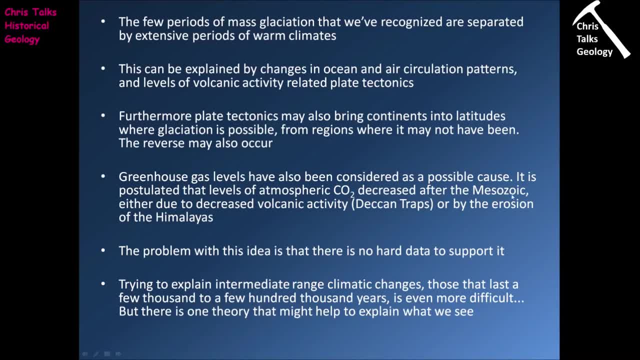 Now we know that carbon dioxide levels decrease after the mesozoic, and this is either due to a decrease in volcanic activity, because for a larger period of time during the mesozoic we have the decantrap flood, basalt eruptions of India, and these huge volcanic eruptions would have pumped out absolutely vast quantities of carbon. 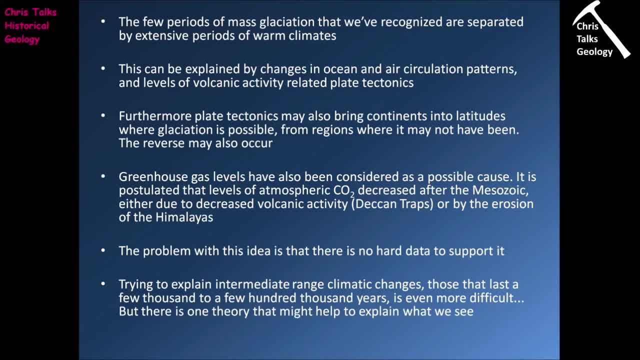 dioxide, and so that would have helped to increase the greenhouse effect. Now, as we transition from the mesozoic into the cenozoic, the decantrap eruptions stop. At the same time, we also have India beginning to interact with Asia, forming the Himalayas, and this occurs about. 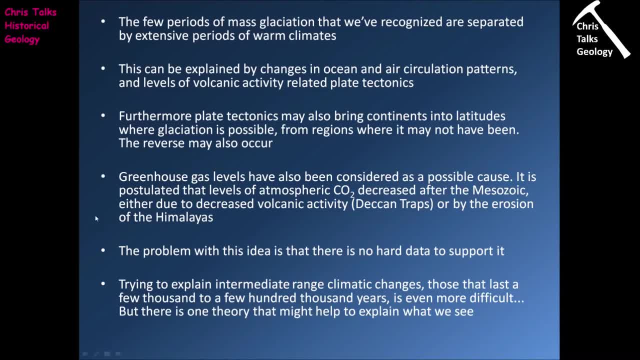 50 or so million years ago, And what we see occurring when the Himalayas begin to form is we obviously see an increase in the rate of erosion and, as part of the erosional process, one of the chemical reactions that can take place is you can have carbon dioxide from the atmosphere. 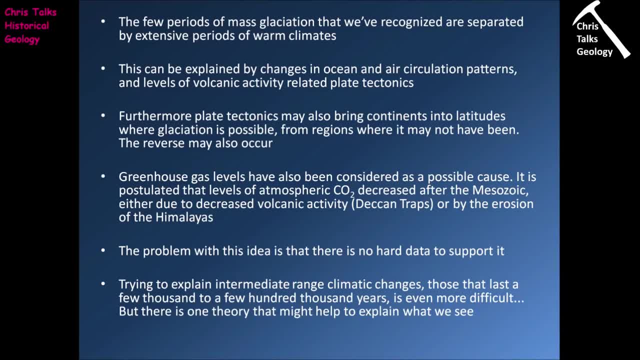 reacting with water and calcium-bearing minerals, and that can lead to the formation of calcium carbonate, And so the formation of a large mountain range like the Himalayas, and the high rates of erosion which are associated with those large mountain ranges can also help to strip carbon dioxide from. 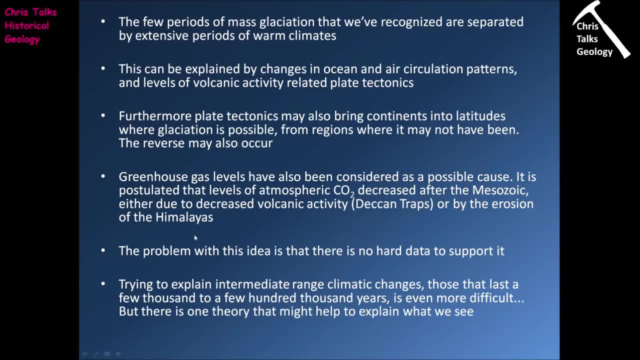 the atmosphere. So both of these factors combined would have been sufficient to have caused a decrease in global carbon dioxide levels and therefore a decrease in the greenhouse effect. So that would make a lot of sense as a possible cause for the onset of the last ice age. 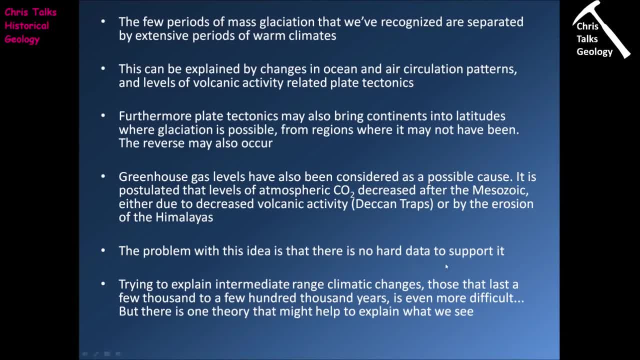 The problem is is that there's no hard data to actually support that idea. So it's not like we see the carbon dioxide levels dropping and then straight away bang, we have an ice age starting. It doesn't work that way. We don't see that in the rock record, and so 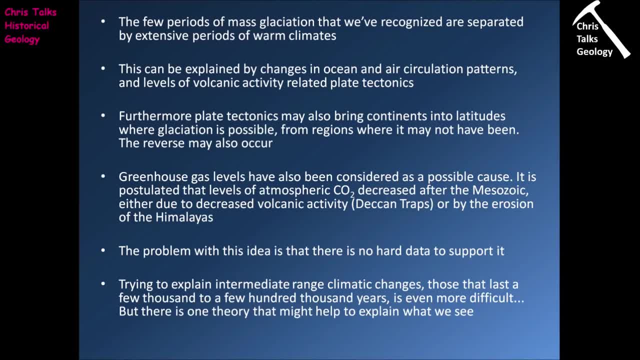 that would suggest that maybe the greenhouse gas levels are playing a part, but it's clearly not the only cause. There must be other factors operating which are also having an effect. So trying to explain intermediate range climate changes, so those that last a few thousand years, 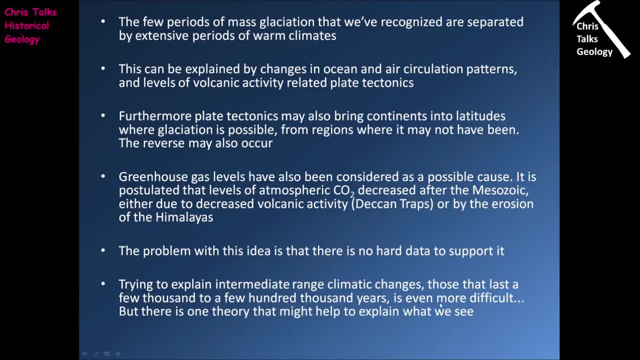 to a few hundred thousand years is even more difficult. So we can explain the big changes. you know we can explain them based on things like changes in ocean circulation and changes in atmospheric greenhouse gas levels, but on the smaller time scale, trying to explain, 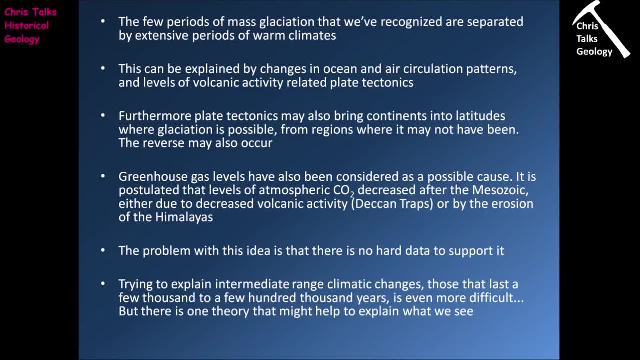 you know, relatively short-lived changes in climate, on both local and global scales, is even more complicated, and so, as you can see, it's a very difficult problem because there's just so many variables. now there is one theory that to some degree does help to explain the onset. 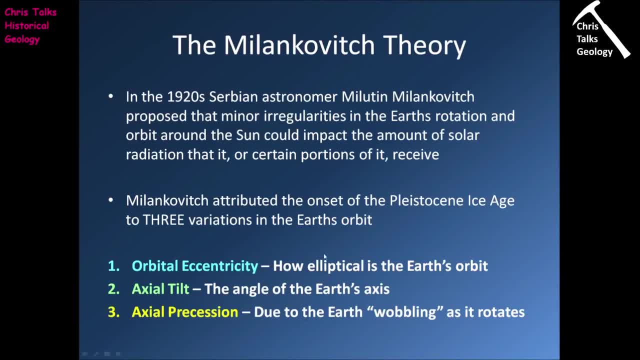 of glaciations. so this is called Milankovic theory. so it was proposed in 1920 by a Serbian astronomer and his proposition was that minor irregularities in the earth's rotation and orbit around the sun will impact the amount of solar radiation that the earth or certain portions of the earth 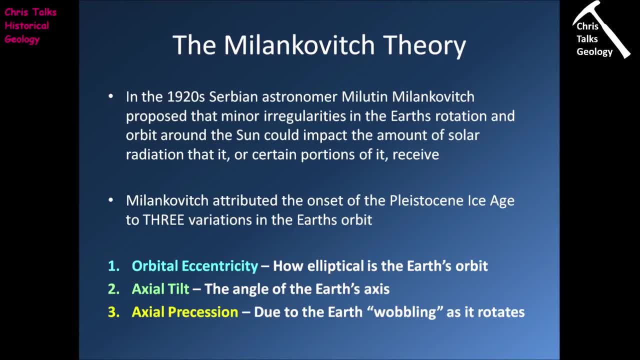 will receive on a yearly basis, and so what he's saying is is: you know, if you manage to reduce the amount of solar radiation an area of the earth's surface is receiving, that's going to result in a cooler climate. Now Mankiewicz attributed the onset of the Pleistocene Ice Age 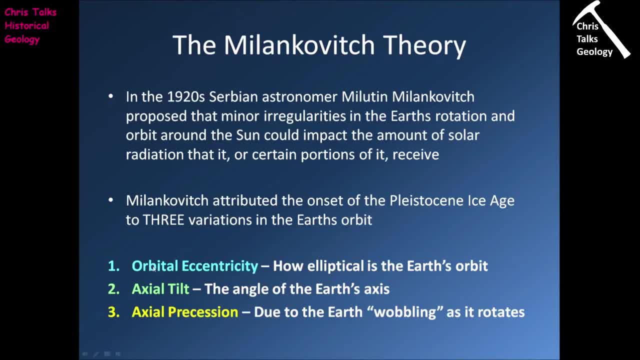 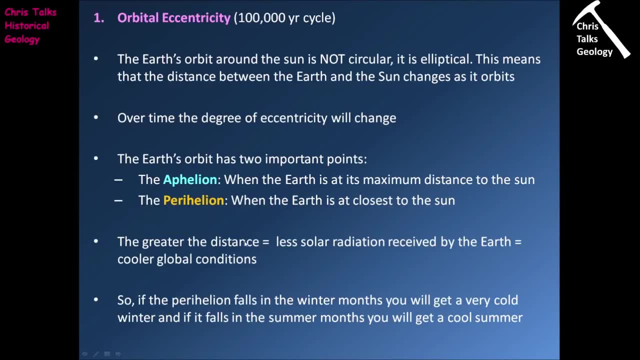 to three variables in the earth's orbit: the earth's orbital eccentricity, its axial tilt and its axial precession. Okay, so let's start thinking about orbital eccentricity now. this one works on a cycle of about 100,000 years, so the earth's orbit around the sun is not circular, it's actually. 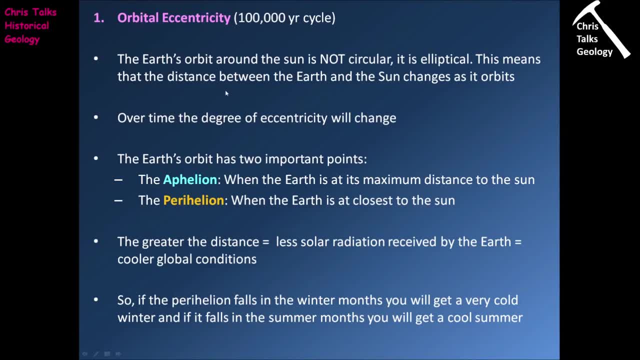 elliptical, and this means that the distance between the earth and the sun will change as it orbits around. Now, over time, the degree of eccentricity will change, so sometimes the earth's orbit is more circular and sometimes it's more elliptical, and these changes will happen on a 100,000 year time. 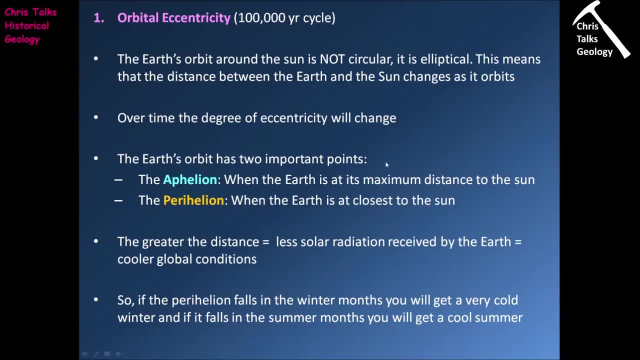 scale. Now the earth's orbit has two important points: the aphelion, and this is when the earth is at its maximum distance from the sun, so that's its furthest point from the sun during its orbit. and then we have the periphyllium. 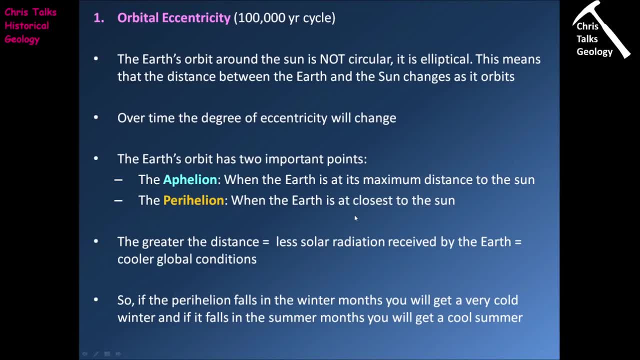 This is when the earth is at its closest point to the sun as it orbits around. Typically, the greater the distance, the less solar radiation will be received by the earth and the colder the climate will be. So if the aphelion falls in the winter month, so that's the greatest distance between the 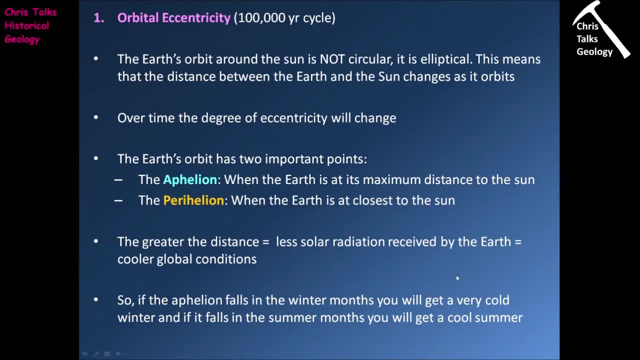 earth and the sun. the earth will obviously be receiving less solar radiation, and so this would result in a cold winter. In contrast, if the aphelion falls in the winter month, the earth will uh if the peri. if the aphelion, sorry, falls in the summer months, you will end up getting a cool summer. 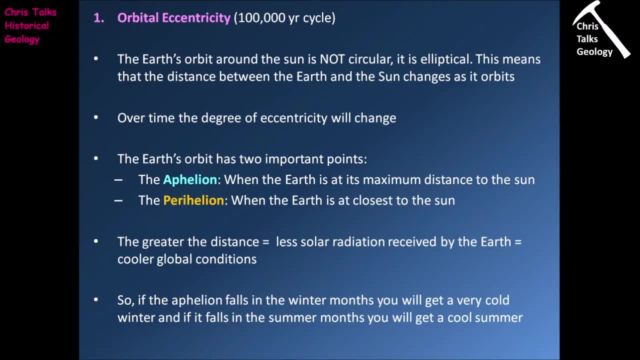 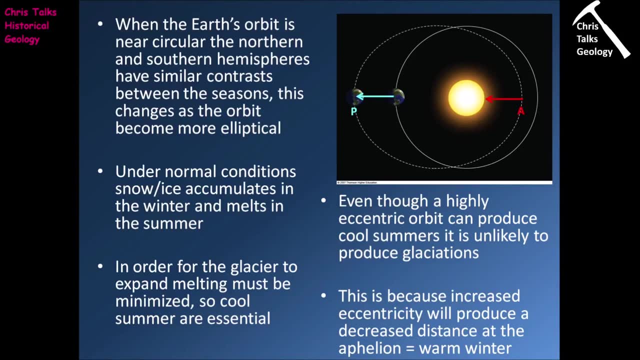 because you'll be receiving less solar radiation. so you can see how this would begin to have an effect now, when the earth's orbit is near circular, the northern and southern hemispheres have similar contrasts between the seasons, and this will change as the orbit becomes more elliptical. so if we look 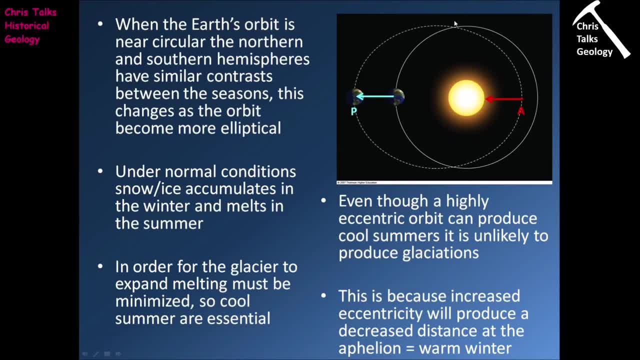 over here. at this diagram you can see we have two orbits: a solid white line, which represents a circular orbit, and a dashed white line, which represents an elliptical orbit. so let's just think about how the seasons would vary between these two different orbits. so let's just say over. 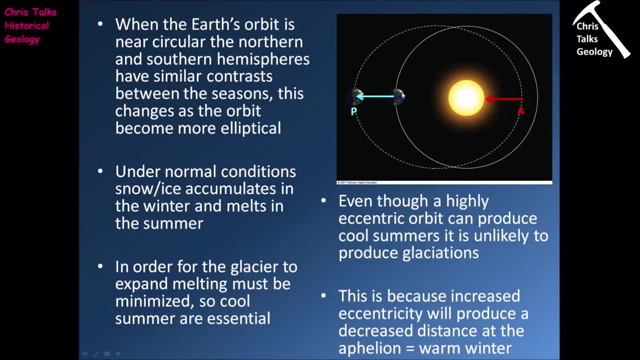 here this represents the northern hemisphere summer, and so over here we would have the southern hemisphere summer. now, because the distance is the same on both sides, it means the summer conditions for the northern and southern hemisphere would be the same, and that would also go for the winter. 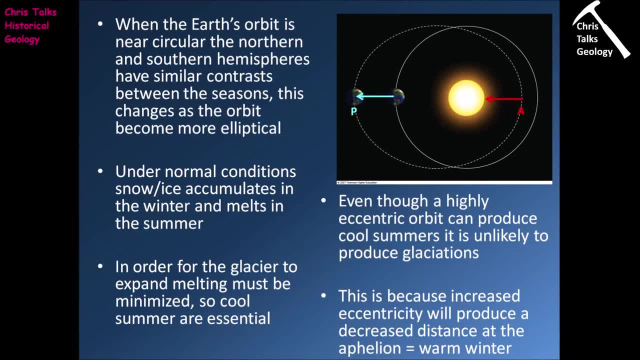 conditions. so you would have very similar conditions between both north and the southern hemisphere. so the the northern hemisphere summer would be very similar to the southern hemisphere summer and the southern hemisphere winter would be very similar to the northern hemisphere winter. now, as the orbit becomes more elliptical, this situation changes. 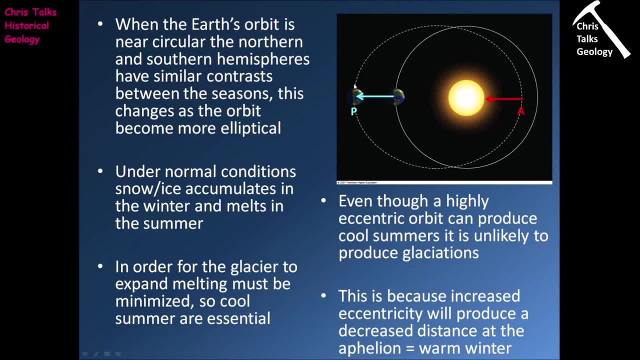 so let's just say, for instance, we have a situation where this represents the northern hemisphere summer. well, obviously, we're a very long way from the sun at this point. so in the northern hemisphere we're going to have a very cool summer, and in the southern hemisphere we're going to have a very cool winter. 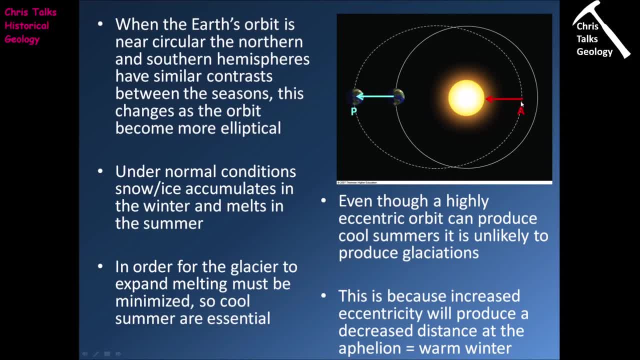 when the earth is on the other side. we would have a very, very warm winter for the northern hemisphere because we're so close to the sun, and we would have a very warm summer in the southern hemisphere. so the the difference between the seasons between the northern and southern hemisphere would be. 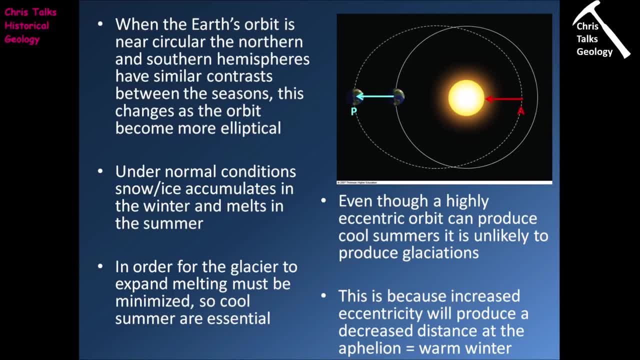 a lot more pronounced now. typically, what this means is: the greater the difference between the winter and the summer, the typically the more snow will accumulate in the colder winters and the more snow will be lost in the warmer summers. now, under normal conditions, the ice and snow will accumulate in the winter and it melts in the 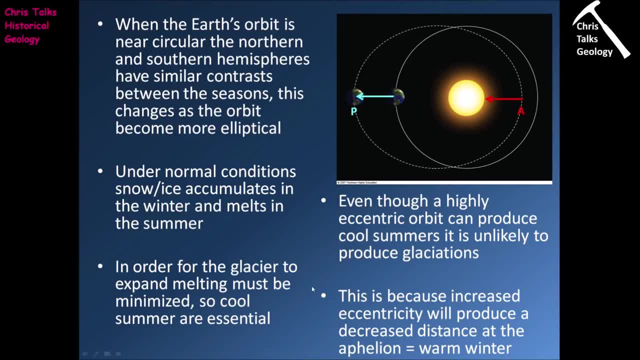 summer. that's not a huge surprise. now, in order for a glacier to expand, we actually want to focus on minimalizing the melting. so what we really want are cool summers. so one of the things that people don't realize- and until you've lived in a very, very cold area, like Canada, for instance- is that 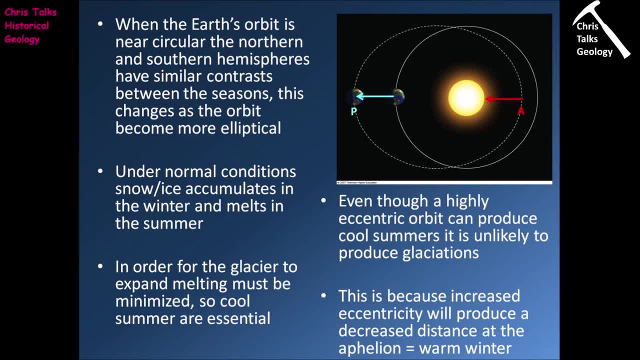 it's very, very cold, it actually inhibits the capacity of snow to form, and so very, very very cold winters will actually result in lower snowfalls. typically, you want your winter to be a little bit towards the warmer end, and this will help to encourage large amounts of snow to. 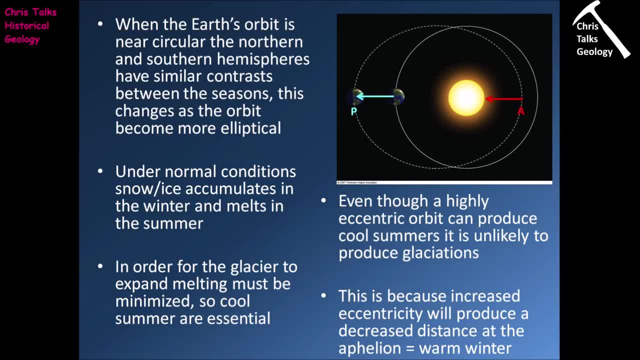 form. now, obviously, what we don't want is a nice, warm summer, so typically what we want is a relatively cool summer and a likely warmish winter, and both of those factors combined will result in heavier snowfall in the winter and less snow melting in the summer. now, obviously this means that when we have a situation 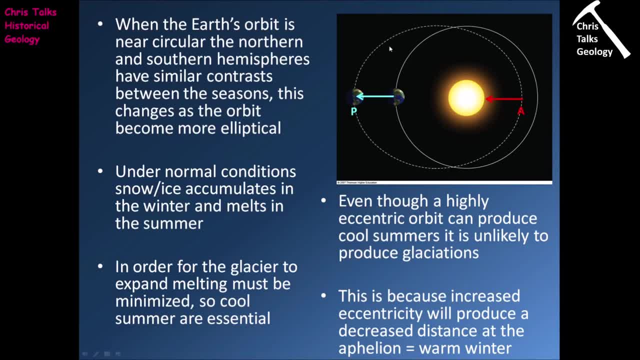 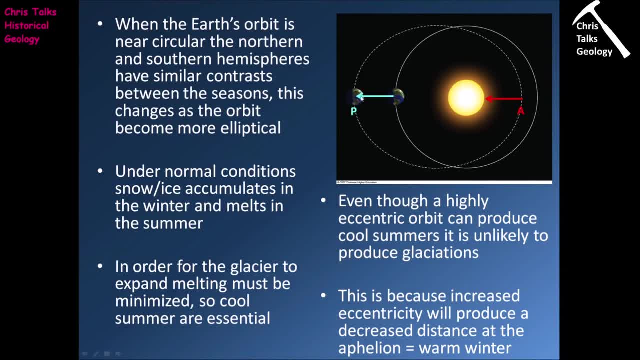 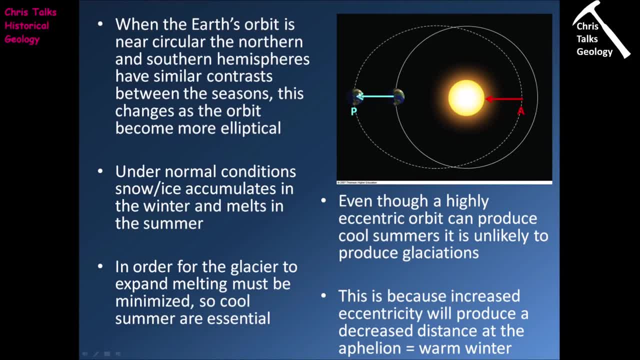 the northern hemisphere, and so the distance between the sun and the earth is obviously the greatest summer months we're going to get a nice cool summer now. that's good for glaciers. however, when we're over here we can see the earth is going to be at its closest to the sun. 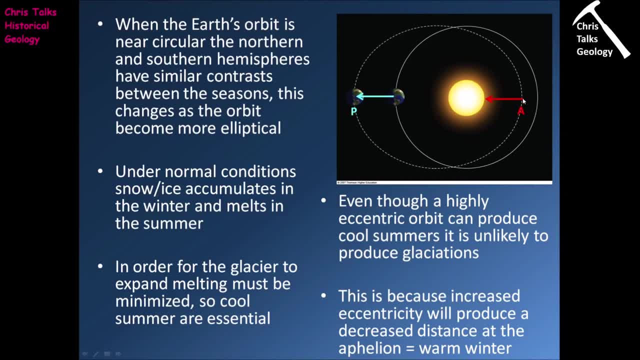 so this would be the northern hemisphere winter. so in this situation we might end up with with a very, very warm winter, and a very warm winter is obviously going to stop snow deposition. it's going to mean that any snow that gets deposited will melt, and so that's going. 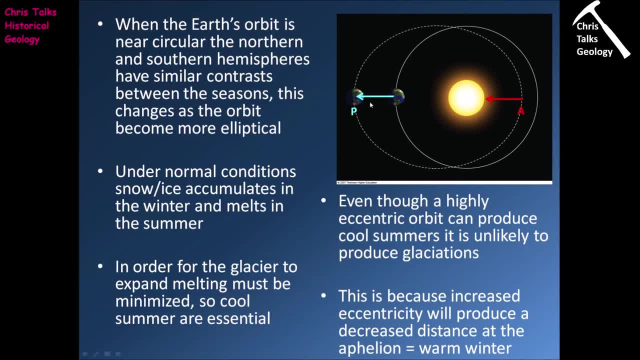 to inhibit glacial formation. let's think about this the other way. then let's pretend that this is the northern hemisphere winter over here. well, in this case we're going to have a very, very cold northern hemisphere winter, and that might actually inhibit snow deposition when we come over to the 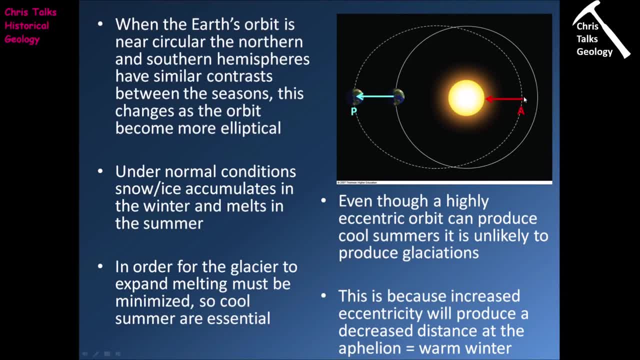 other side, we're going to have a very, very warm summer and obviously that's going to cause lots and lots of melting. so you can actually see that very elliptical orbits are actually bad for glaciations. what you want is an orbit that's kind of somewhere in between a circular orbit and the most extreme. 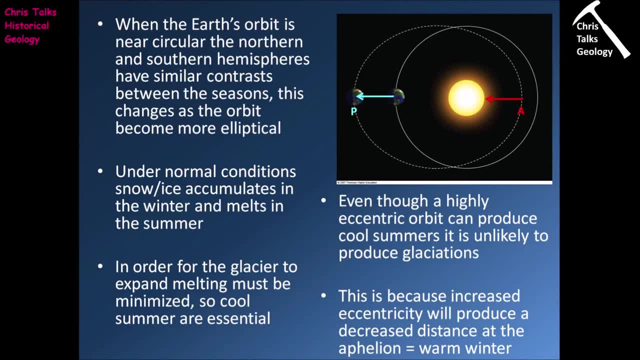 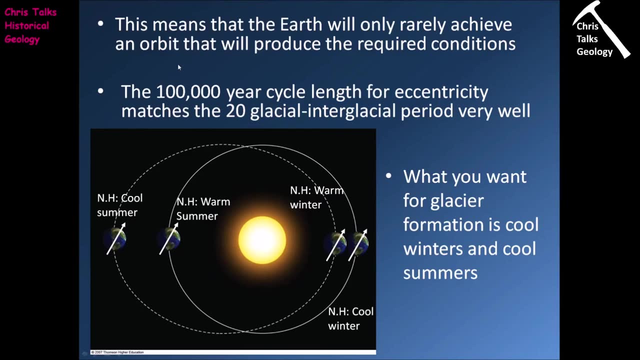 elliptical orbit, because that's going to offer you a good contrast between the seasons, but at the same time the seasons aren't going to be too extreme now. this obviously means that the earth will only rarely achieve the kind of orbit required to produce the conditions we want for a large-scale glaciation. so the 100,000 year cycle length for 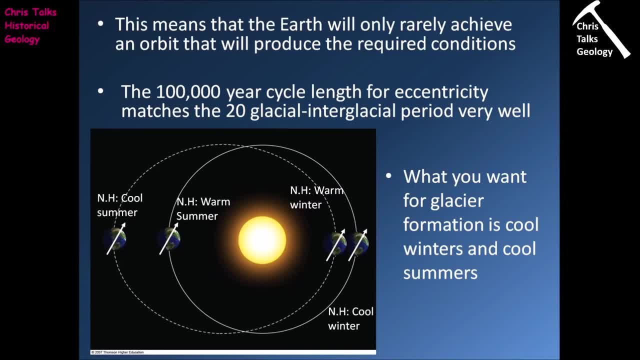 eccentricity matches very, very nicely with the 20 interglacial periods which we have from the, from the Pleistocene. so obviously we have 20 interglacial periods, we have a cycle of 100,000 years. that's going to equate to approximately 2 million years of time, and we know the last ice. 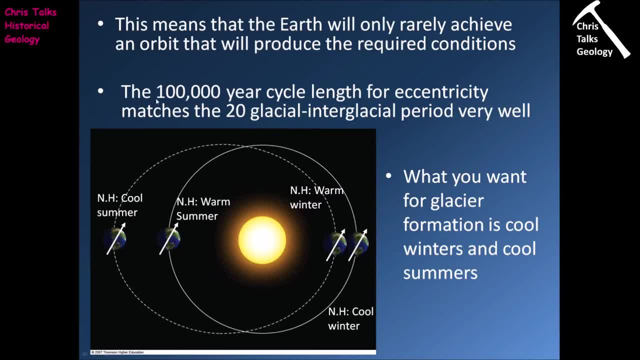 age was about 2.6 million years, so this equates absolutely wonderfully. so essentially, what it comes down to is, what we really want is an orbit that's going to encourage relatively cool but not excessively cold winters and cooler summers that's going to encourage relatively cool but not. 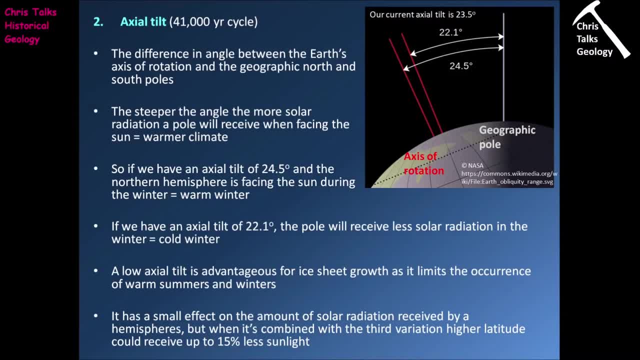 what we really want. so our next variable is axial tilt, and this operates on a 41,000 year cycle. so the axial tilt is the difference in angle between the earth's rotation of axis of rotation and the geographic north and south poles. the geographic north and south poles are simply put: 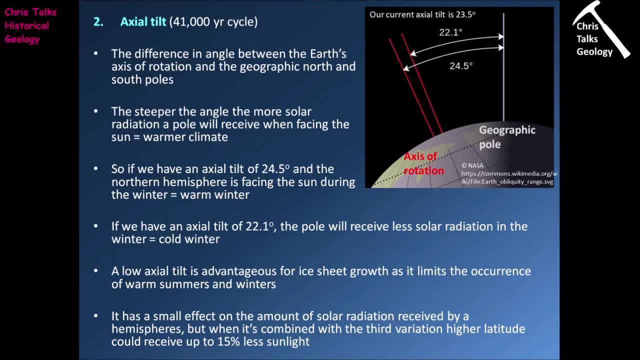 there by map makers, and those are essentially the poles that stick out at the top and the bottom of the earth. in reality, the earth doesn't actually rotate around the geographic poles. it rotates along the axis of rotation, and the axis of rotation is actually offset from the geographic north and south poles and the axis of rotation. 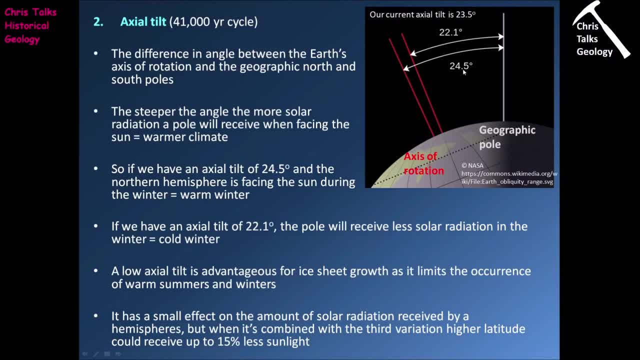 can be anywhere between 22.1 and 24.5 degrees off the geographic north pole. at the moment, our current tilt is about 23.5. now, the steeper the angle, the more solar radiation a pole will receive then. this is because the steeper the angle, the more of the pole will be exposed to the sun, and so 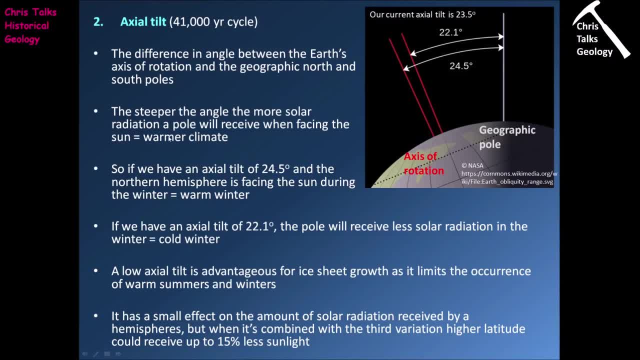 the more solar radiation the area receives, the warmer the climate will be. so if we have an axial tilt of 24.5 degrees and the northern hemisphere is facing the sun during the winter, well, this would mean we would have a very warm winter. now, if the axial tilt is 22.1 degrees, so the lowest angle, your total aren't too high. in the air pour both miles verloren out. the temperatures are above expectations. the pole will receive less solar radiation is a very long area, so in the near квартиance of hot weather this is an area pointing to the south, at 24.5 and to heat it's all Orange. your area is a veiled Dirichlet. 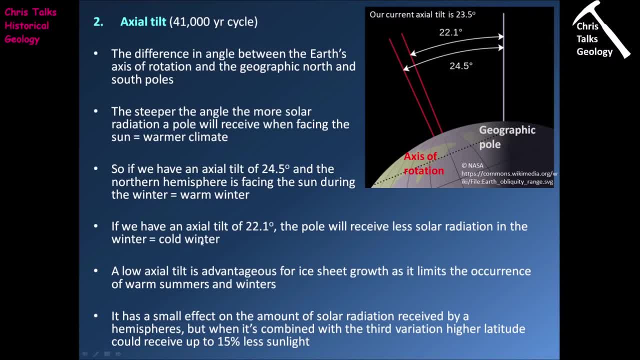 there's actually a high temperature on south the working system. this means that are solar radiation as of radiation in the winter and this would actually result in a cold winter. so you can see pretty quickly what we want is we want our axial tilts to be as low as possible. 22.1 is the number we're. 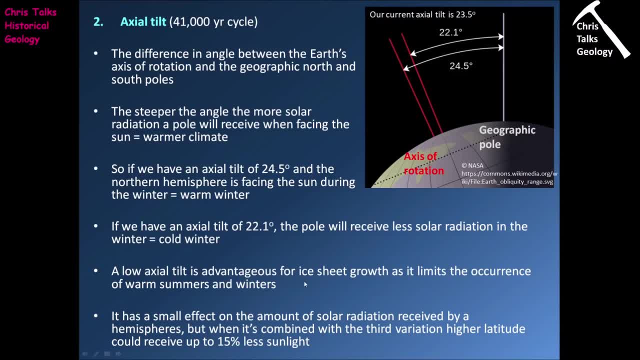 really looking for. so a low axial tilt is advantageous for ice sheet growth as it limits the occurrence of warmer summers and winters. so typically, the lower the angle, the cooler. the warmer- sorry- the cooler the summers and winters will be, so the effect of the axial tilt is actually quite. 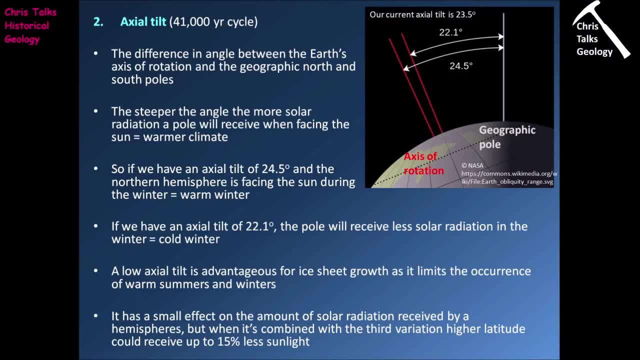 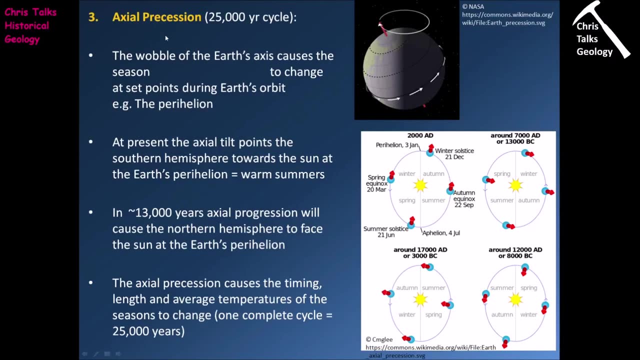 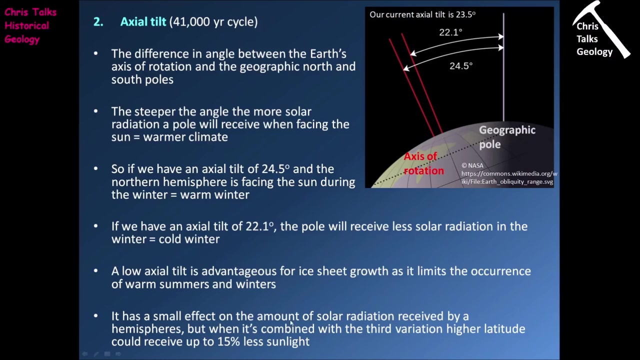 small. however, the combined effect of the axial tilt and the next variable can actually lead to a change in solar radiation levels of up to 15. so when we combine axial tilt and axial precession together, it can actually reduce the amount of sunlight received by a pole by up to 15. 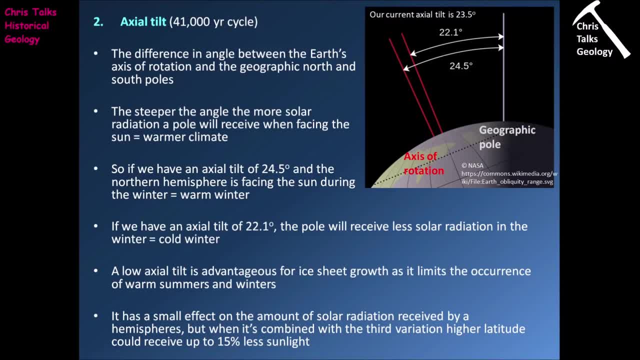 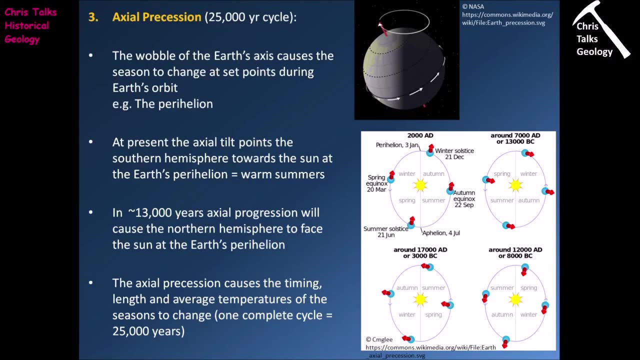 and obviously the less sunlight we have, the less solar radiation we have hitting the pole, the, the the rotates. you can see, if we look at this diagram, that the axial plane doesn't actually stay stable. instead it rotates in a circular motion and this actually produces a wobble in the earth's 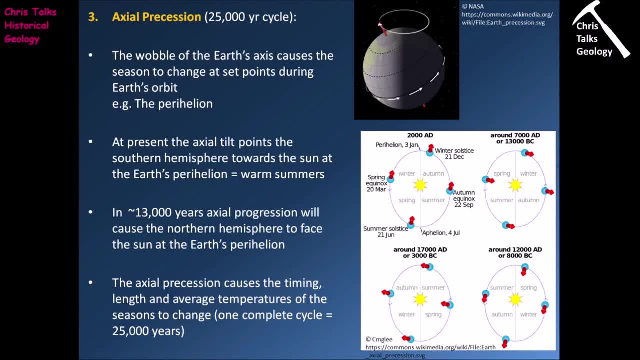 rotation. now, what this means is the tilt of the earth will change over time. so you can see in this picture the axis of rotation is orientated northwest- southeast. however, given enough time, the axial plane will actually come over here and the axis would then be situated in a northeast- southwest orientation. so you can see. 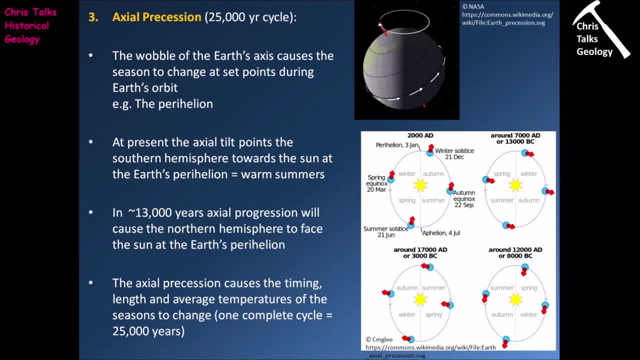 over time the angle of the rotation of axis will be changing. now, if we look at this diagram down here, this is actually going to demonstrate what changes this will produce. so if we look here, you can see we have four scenarios where we have the earth orbiting around the sun. obviously the sun is. 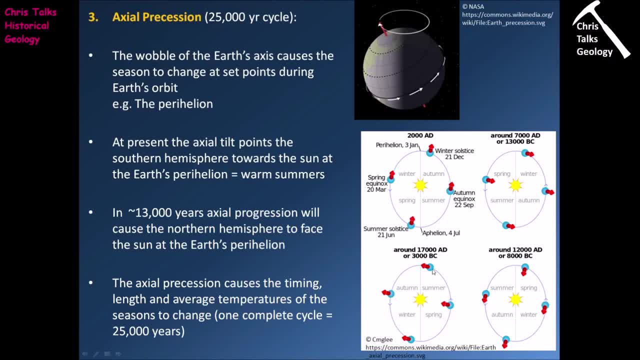 the, the yellow dot in the middle, and the earth is represented by these blue circles, and the red line here is representing the earth's axis of rotation. so what we can see here is that we are looking at the northern hemisphere, and so we can see- in this instance we can see- the axis of rotation is. 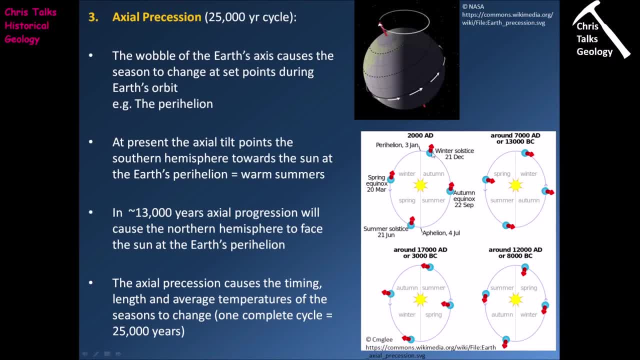 pointing the northern hemisphere to the north hemisphere, and so we can see, in this instance, the axis of rotation is pointing the northern hemisphere away from the sun, so this means we're going to get colder conditions. so this is going to be either the fall or, as we are over here, the 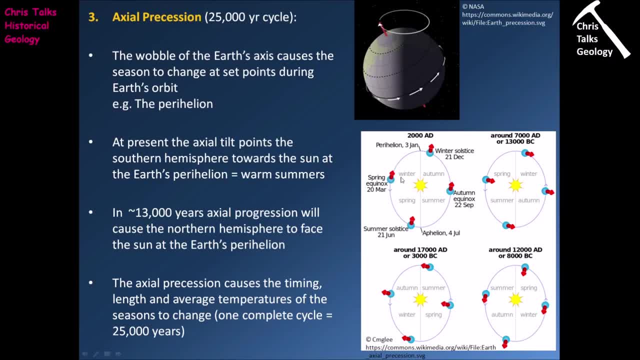 winter. so as the pole is facing axis of rotation is facing away from the sun, that means less solar radiation from the northern hemisphere and that's going to lead to colder conditions. now during the spring months and the summer months, we can see the axis of rotation is going to be pointing the 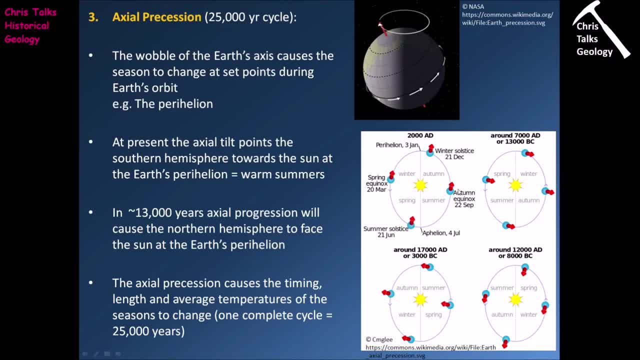 northern hemisphere towards the sun, and this is going to result in warmer conditions, so not really a huge surprise there now. what you're going to notice, though, is that, as we look through earth history, we can see that the position of the axis of rotation has been changing, so this goes back. 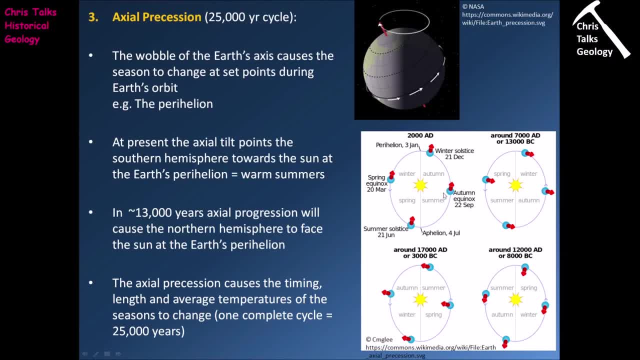 from about 12 000 years ago, the end of the last ice age, through to the present day, so at the end of the last ice age. we can see that at this point here, where in the modern day we have cooler winter, ish conditions, so fall and winter conditions, 12 000 years ago we would have had more spring. 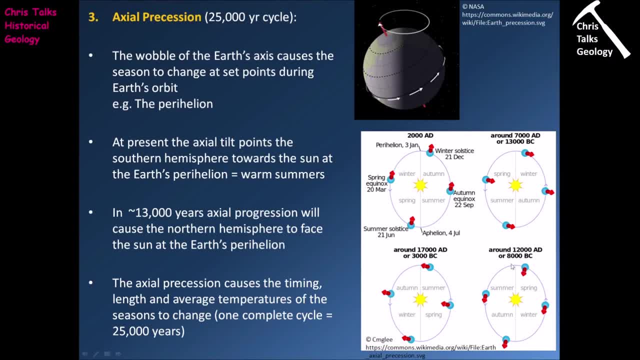 like conditions. it would have been warmer. so you can see that conditions where we are in the spring and summer in the modern system would actually have been autumn and winter about 12 000 years ago. so you can see how this wobble and its effect on the earth's axis of rotation is going to have a quite substantial it's going to cause. 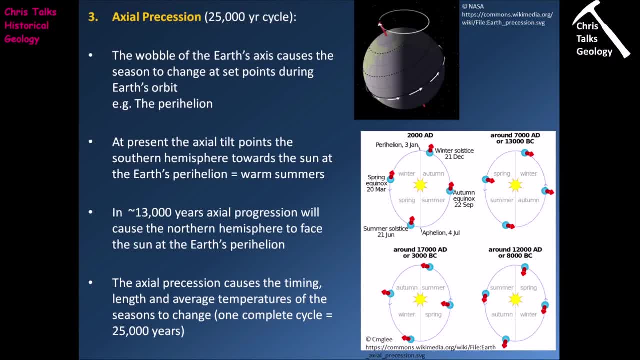 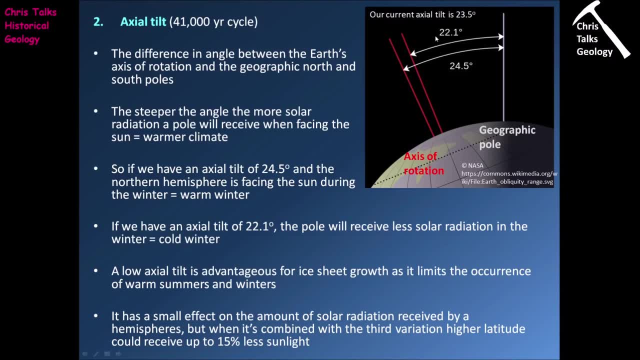 quite substantial changes in the amount of solar radiation received by a pole. now, when you combine that with the change in axial tilt- if you can get a 22.1 degree axial tilt- and combine it with a situation where we have the earth's axis of rotation- 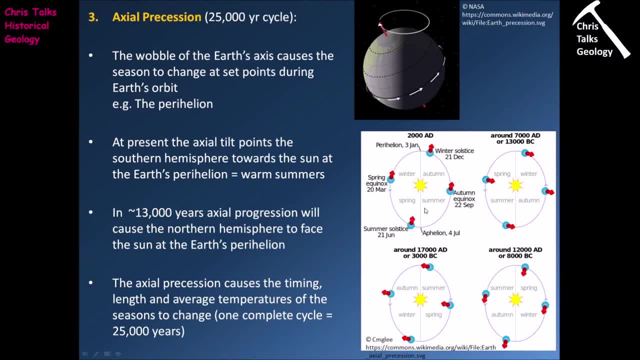 facing away from the sun in the spring and summer. well, that would obviously lead to quite cold springs and summers and that would be quite good for glacial formation. now, at present the axial tilt points the southern hemisphere towards the sun at the earth's perihelion, so essentially that means the southern hemisphere has nice, warm summers. now, in about 13 000 years. 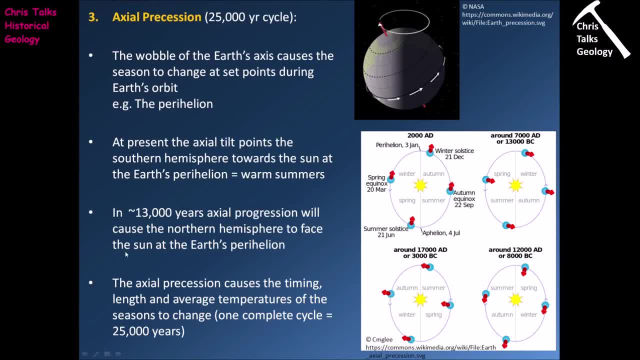 precession is going to cause the northern hemisphere to face the sun at the earth's closest point, and so this means in about 13 000 years time we are going to be having very, very warm winters in the northern hemisphere. so the axial precession causes the timing, the timing. 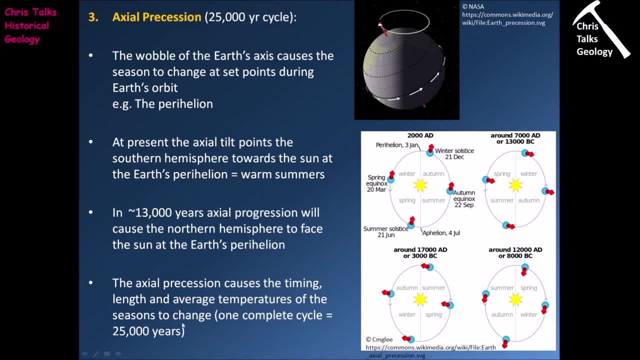 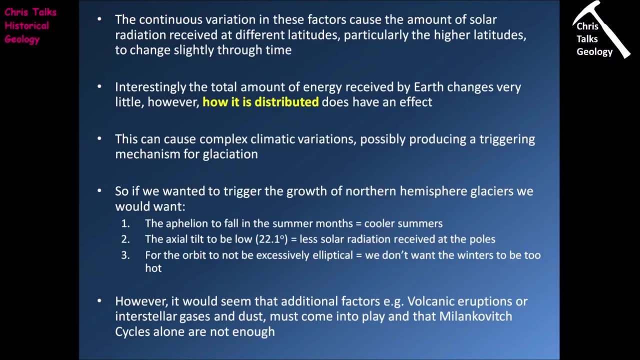 length and average temperatures of the seasons to change, and one complete cycle will take about 25 000 years. so these three factors combined are obviously going to result in changes in the amount of solar radiation received by certain parts of the earth's surface. now, the continuous variation. 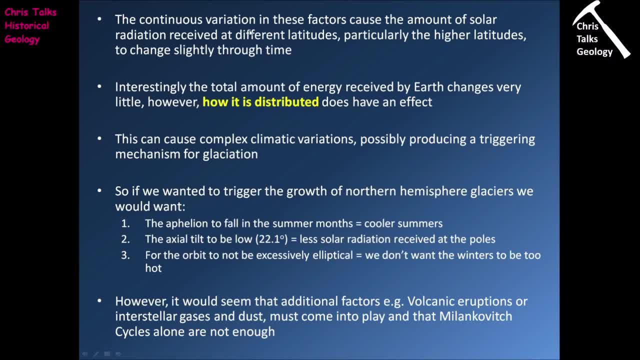 these factors causes the amount of solar radiation received at different latitudes, particularly the higher latitude, so towards the poles- to change slightly through time. interestingly though, the total amount of energy received by the earth doesn't change very much. what we're actually talking about is changing the distribution of the solar energy. 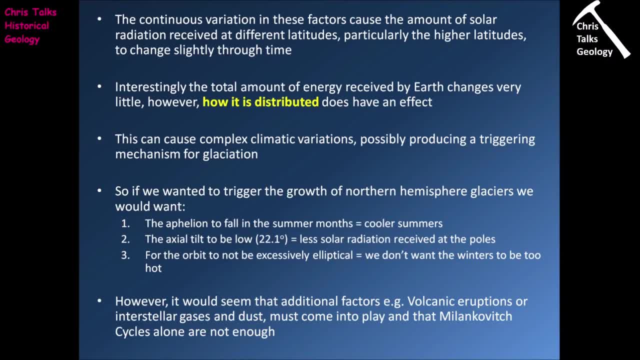 so what we're trying to do is we're trying to change how much solar energy the northern or southern hemisphere receives at certain points of the year. now, obviously, this can cause very complex climatic variations, possibly producing uh, possibly, or triggering a mechanism for glaciation. so the problem is: is that, yes, we have these three variables and, yes, they're going to contribute? 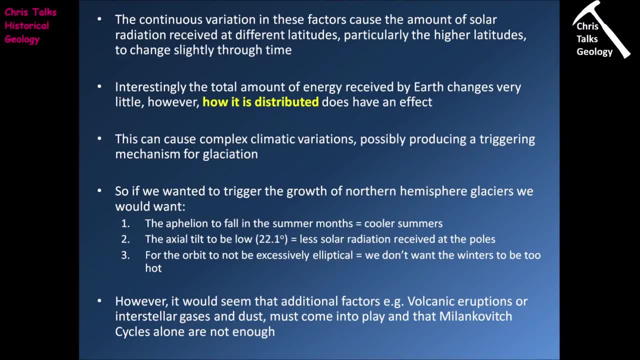 but on top of that we are also going to have the complicating factors of things like greenhouse gases. we're going to have, you know, the effect of global warming related to human beings. you know, we may have other variables which will also affect global temperatures, something like. 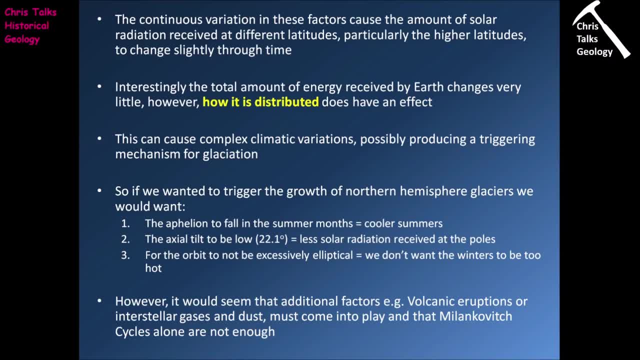 large-scale volcanic eruptions, throwing lots of dust and ash into the high atmosphere, which could cause the global climate to cool down. so the Milenkovic cycles on their own aren't truly going to be sufficient to induce a large-scale glaciation. however, if we wanted to encourage or at least improve our chances of producing a northern 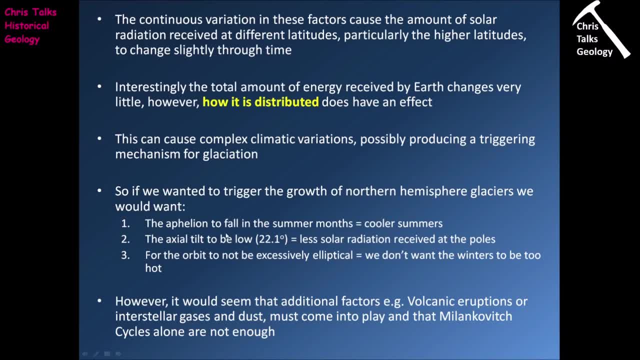 hemisphere glaciation, for instance. what we would really want would be the aphelion to fall in the summer month, which is going to give us a cool summer, so we're going to lose less snow and ice through melting. we want the axial tilt to be low, typically about 22.1 degrees, and this 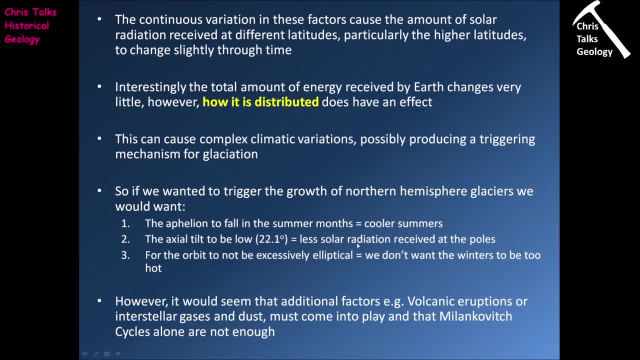 means that we're going to have a lot of snow and ice melting and we're going to have a lot of ice through melting. we want the axial tilt to be low, typically about 22.1 degrees, and this means the northern pole or north pole will receive less solar radiation and, as such, it will be cooler. 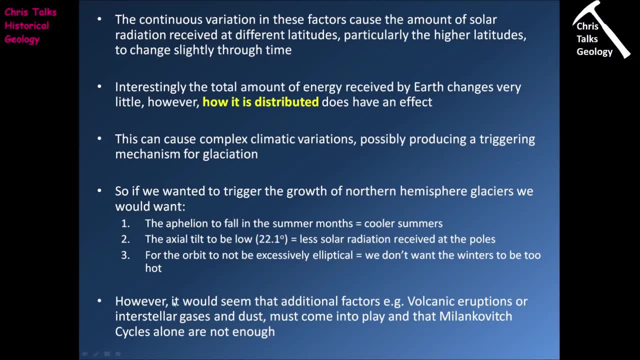 which will once again encourage ice growth. we also don't want the orbit to be excessively elliptical. we want it to be somewhere between a circular orbit and the maximum elliptical orbit, and this means that we get winters which will be not too hot and not too cold. 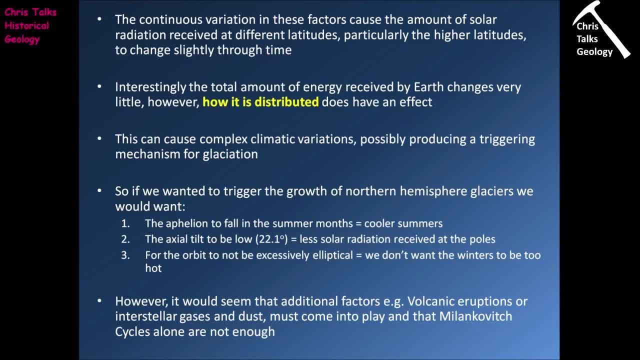 and we'll get summers that won't be excessively hot, and this will encourage the development of snow and ice during the winter period and it will minimize the amount of melting we get during the summer period, and this will lead to a net expansion in the amount of glacial ice. now the thing we need: 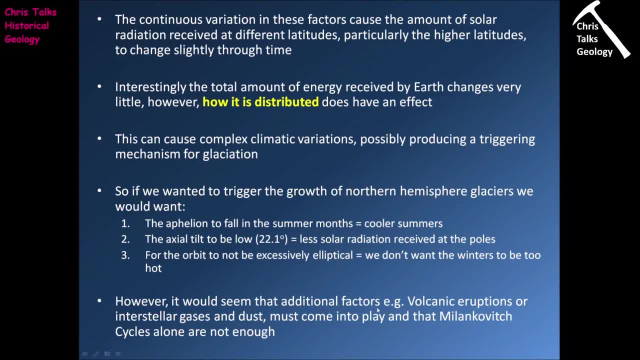 to remember, as I just said, though, is we have to bear in mind that additional factors- so things like volcanic eruptions or maybe the Earth passing through an interstellar dust cloud- can also play a part, so it's not just the Milenkovich cycles alone which are going to control whether we get these mass. 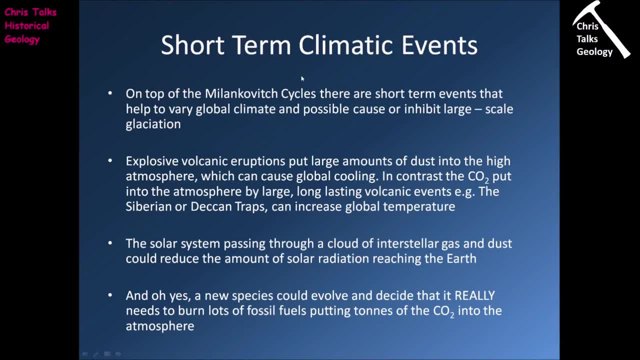 events. So the final thing we need to think about are short-term climatic events and what effect they're going to have. So on top of the Milenkovic cycles, there are also going to be short-term effects that help to vary global climate and possibly cause or inhibit large-scale glaciations. 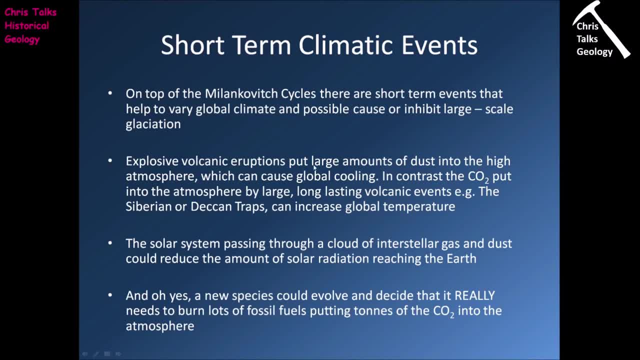 So a classic example would be something like an explosive volcanic eruption that puts large amounts of dust into the high atmosphere. So in 1990 in the Philippines, a volcano called Mount Pinatubo went and erupted. It was a very, very large eruption. It threw lots and lots of dust. 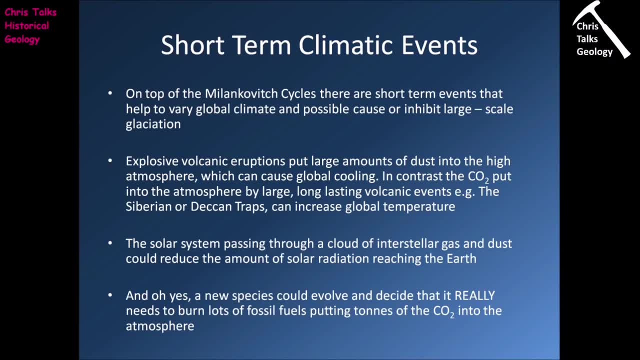 into the high atmosphere. And what this dust does when it enters the high atmosphere is it actually reflects solar radiation back into space. And so for two years after the Mount Pinatubo eruption- so from 1990 to 1992, we actually saw a noticeable decrease. 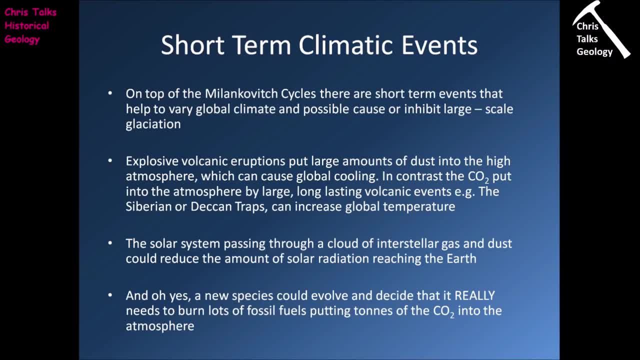 in global temperatures. Now, this was obviously a short-lived event. It only lasted 24 months. In contrast, the carbon dioxide put into the atmosphere by large, long-lasting volcanic events, so something like the Deccan Traps or the Siberian Traps can cause global temperatures to increase. 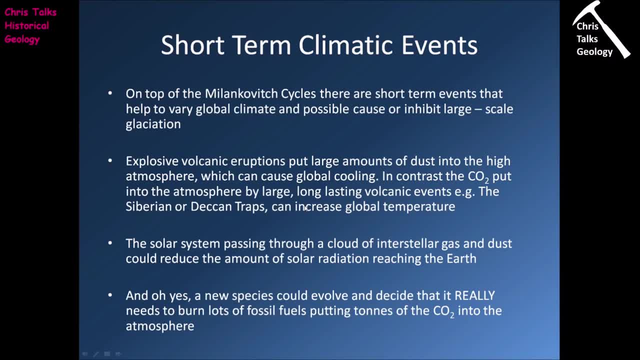 But remember, these large-scale eruptions are going to be operating on a very long time scale, so they're not going to be considered short-term events. Now we can also have events such as the solar eclipse, which is a very long-term event, So we can also have events such as the solar eclipse. 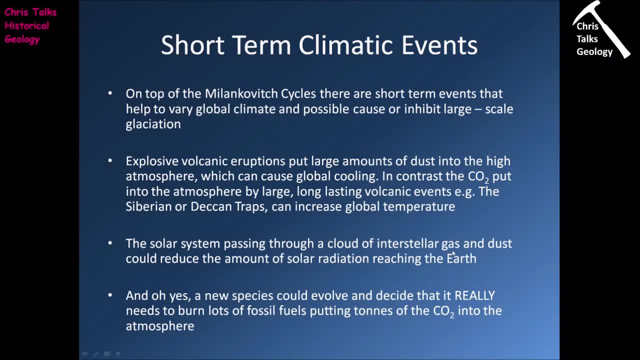 which is a very long-term event. So we can also have events such as the solar eclipse, where the solar system passing through a cloud of interstellar gas. So we always think about our solar system as a relatively stationary thing, but it's not. We're part of a galaxy and that galaxy 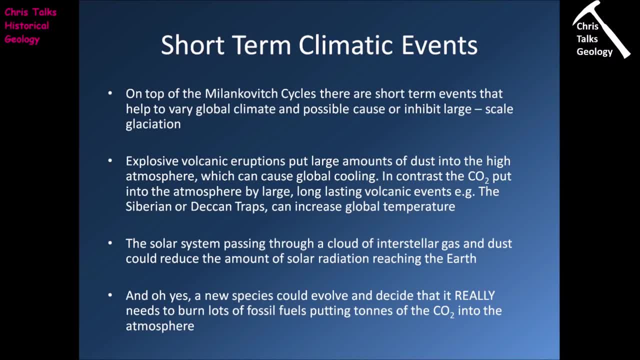 is moving, the galaxy is rotating, and so the solar system is constantly moving through space, And occasionally that means the solar system is going to go plowing through a gas cloud or a dust cloud, And this is obviously going to reduce the amount of solar radiation. the 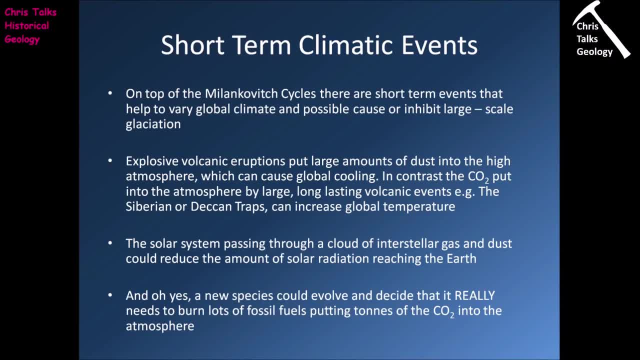 earth receives from the sun because the ash- sorry, because the dust or the gas is going to scatter a certain amount of that solar radiation. So that's going to mean the conditions will get a little bit cooler And of course we can't always overlook the 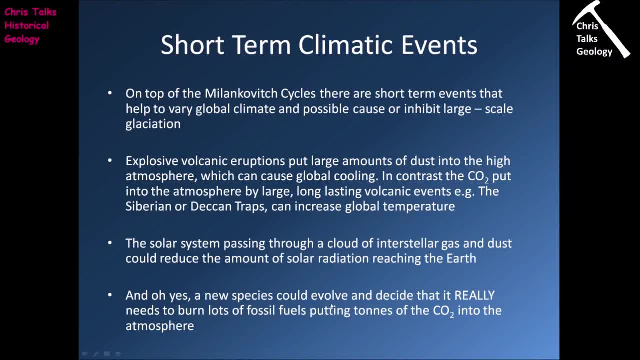 introduction of a new species onto the surface of the earth that decides what they really need to do is burn a whole load of fossil fuels, putting in tons of carbon dioxide into the atmosphere, helping to rapidly increase the greenhouse effect. Yes, we are considered to.